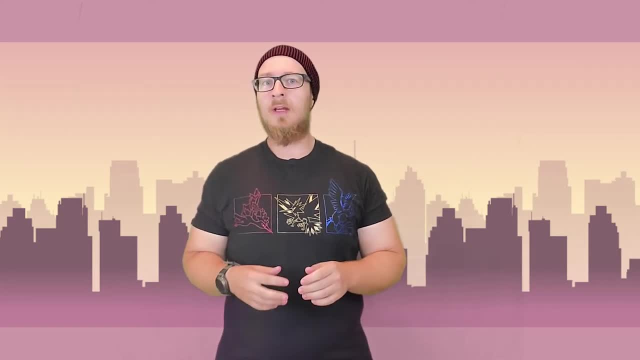 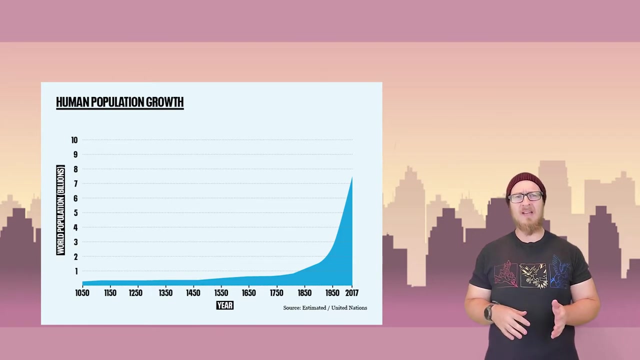 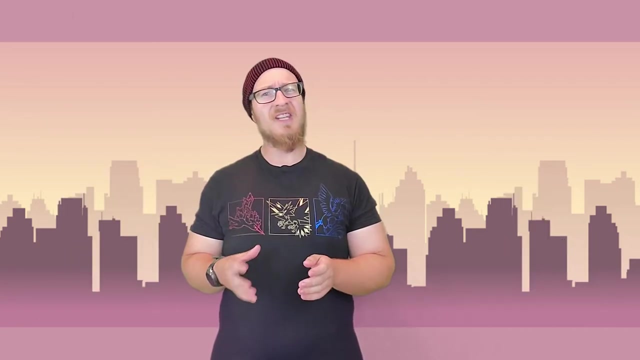 All populations change over time. This is especially true for the most impactful of animal species, the modern human. Human population growth has more or less been exponential since the industrial revolution. This growth, especially today, is not equal in all parts of the world. Let's take a look at the most populated countries as of 2018.. 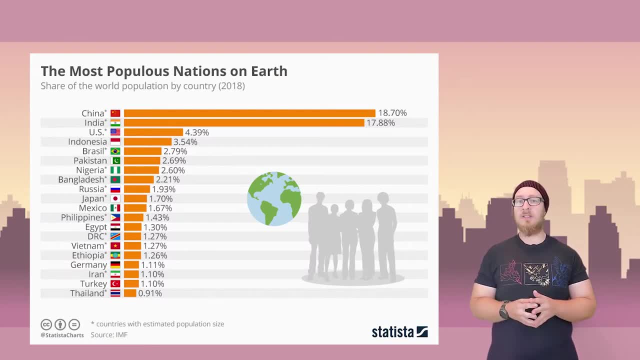 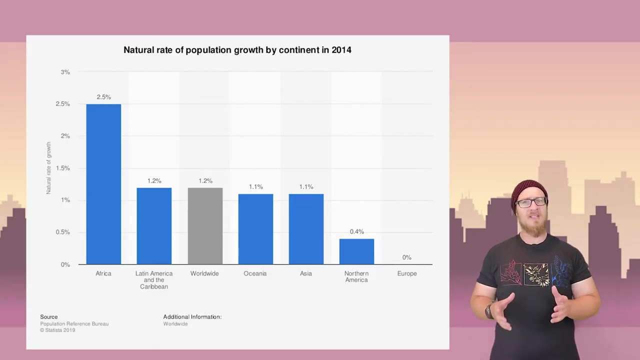 Right now, China, India and the United States are the largest populations by country, with China having the current largest population. The population growth rate, however, right now may change this dynamic. The entire continent of Africa is seeing the largest population. 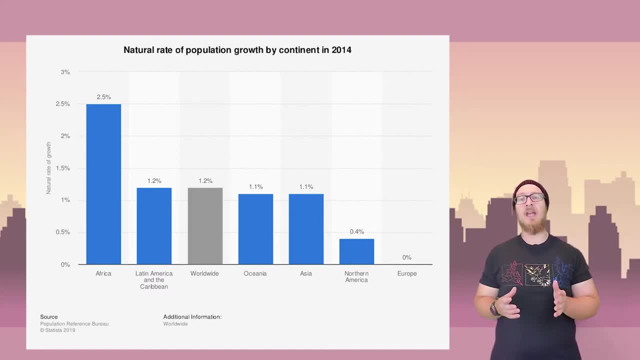 at a whopping 2.5% annual increase. Many parts of Europe, however, are seeing no population growth at all and, as a result, will see a decrease in population in the future. This is also true of North America, which is expected to remain relatively stable. Here's what the global 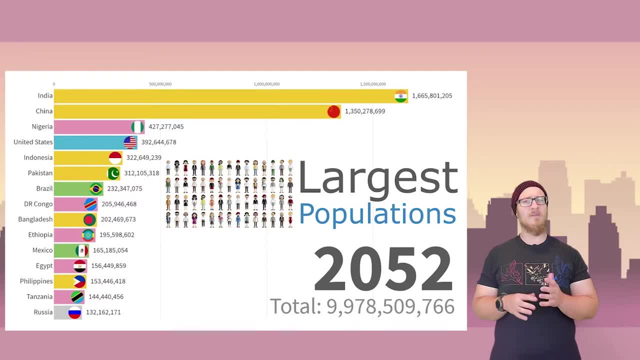 population is projected to be around 2052.. Notice that in the last few years, the population has superseded China as the most populous nation. As expected from the high population growth rates in Africa, the country of Nigeria is expected to have the third largest population in the world. 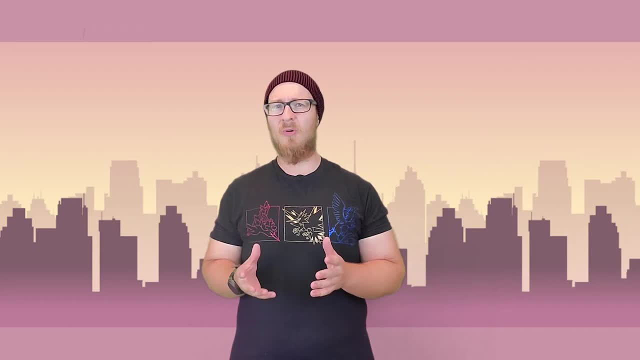 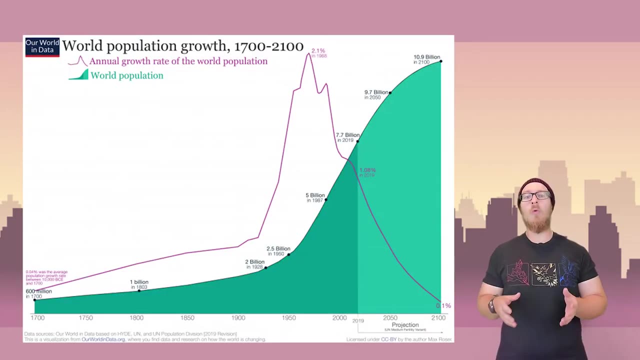 All this growth in population leads to an important question: What is the Earth's carrying capacity for humans? Well, right now, the United Nations believes that the global population will peak in the next few years. The United States believes that the global population will peak in the next few years. The United States believes that the global population will peak. 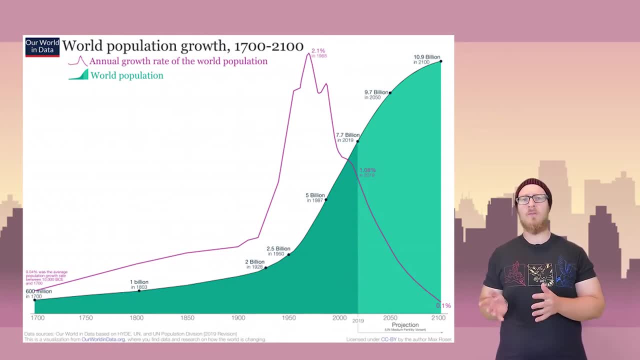 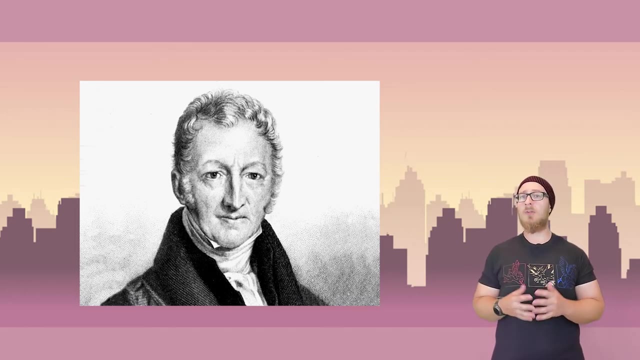 at just below 11 billion near the end of the 21st century and then slowly begin declining. If these projections are accurate, that's a whole extra 3 billion people. In 1798, British economist Thomas Malthus published an essay that, in so few words, claimed that the population growth rate must be controlled, otherwise we'll reach a catastrophic time when disease, war and famine will be a problem. The United States believes that the global population growth rate must be controlled, otherwise we'll reach a catastrophic time when disease, war and famine 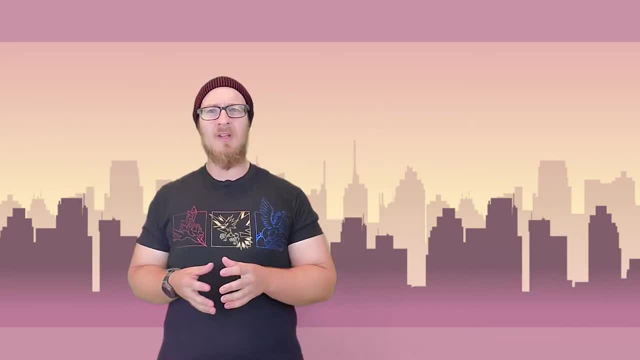 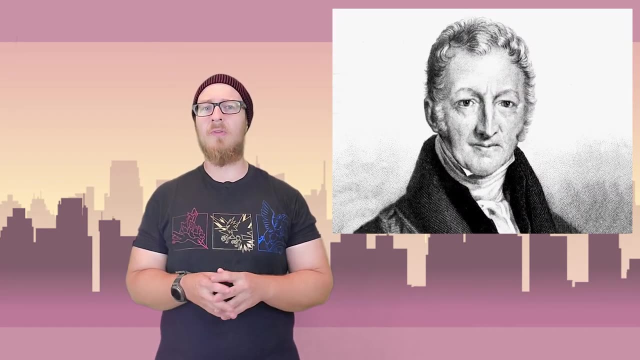 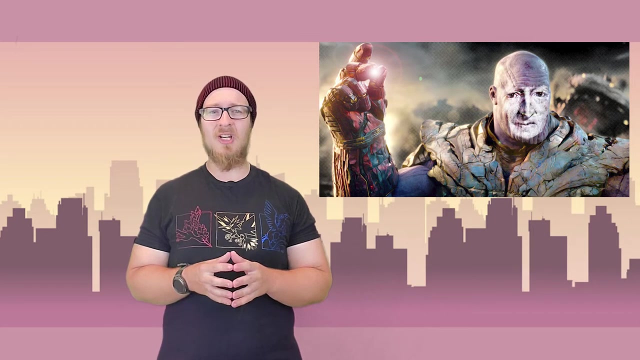 would be the ultimate check. Though he didn't suggest a Thanos approach, he argued heavily for checks on population growth, like abstinence and postponing marriage. Malthus' argument was criticized and his projections have since yet to pass, If the population were to get that high. 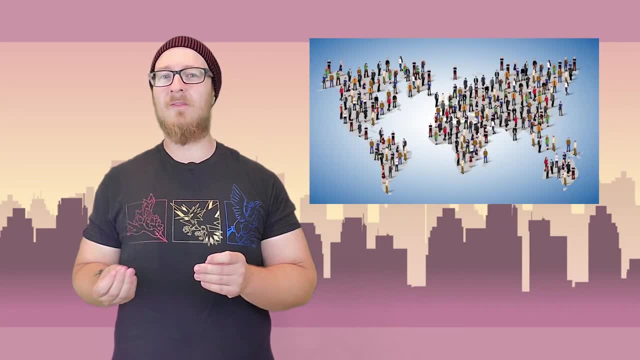 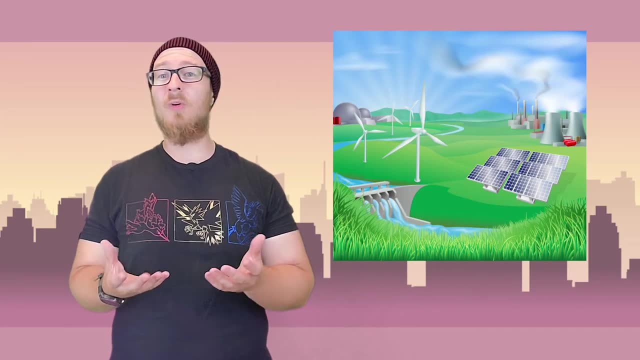 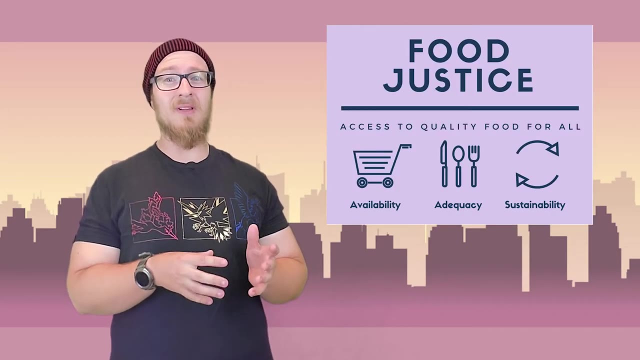 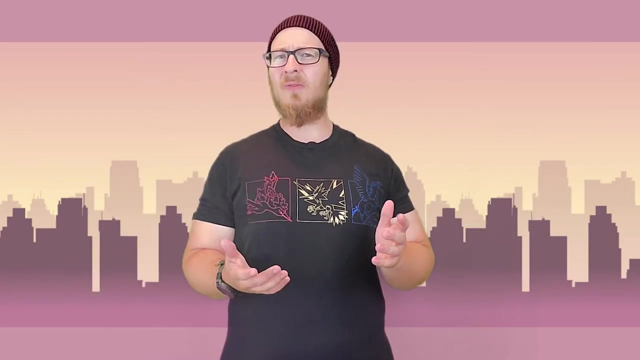 we have to work as a global community if we are to carefully manage global resources. Economically advantaged countries must work to lower their global impacts, especially in terms of carbon dioxide emissions. Further, the growing population will require global cooperation to ensure enough food can be produced. But how can we even make these? 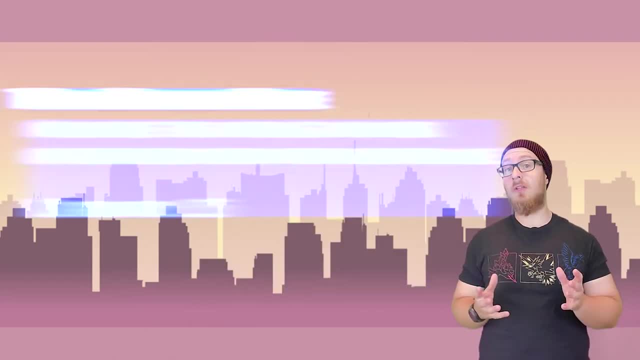 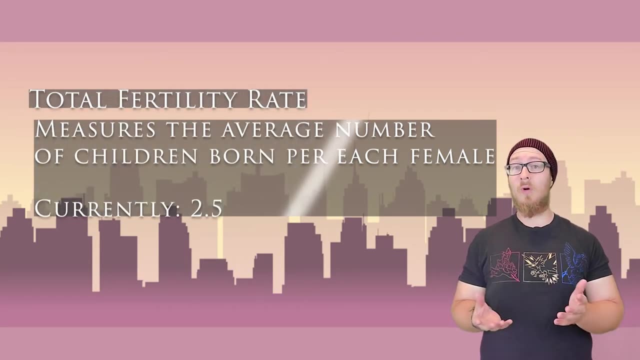 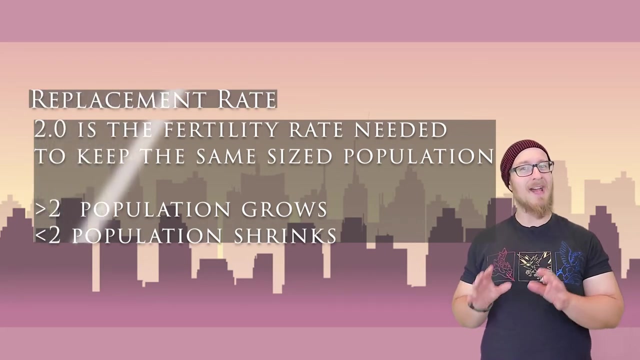 projections. The United Nations looks at fertility rates around the world. The total fertility rate measures the average number of children per woman. Right now, the global average fertility rate is just about 2.5 children per woman. This is above the replacement rate of 2.0.. Now, as we've learned in biology, it takes two people to make a baby. 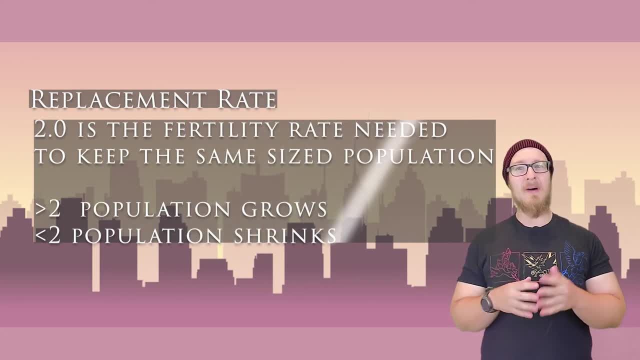 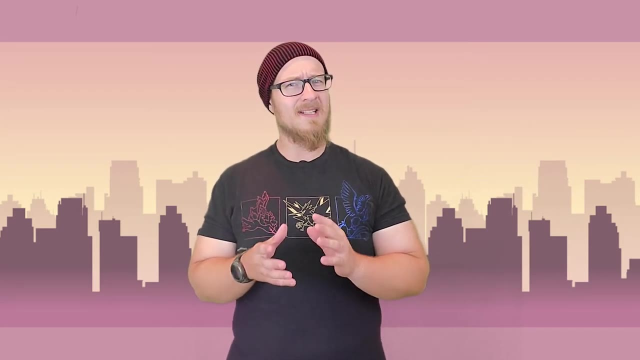 So if two babies are born per couple, the population will remain about the same. Any number above two will see populations increase and any number below two will see the population decrease. That said, the fertility rates can be misleading If there is a high infant mortality rate, even a 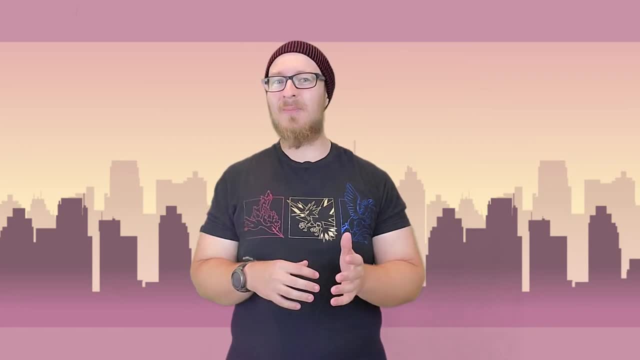 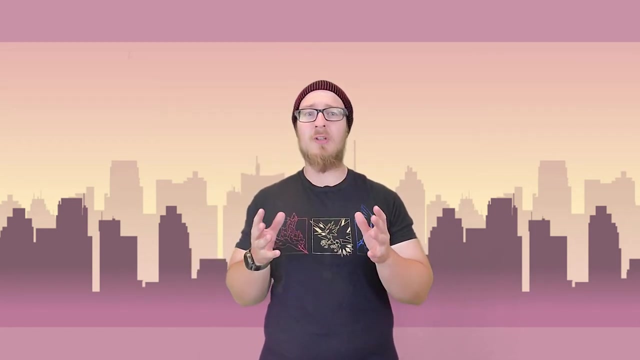 high rate of fertility may still see a stable or decreasing population. One of the leading factors that influences infant mortality rates is whether or not mothers have access to good health care and nutrition. Though there are still disparages globally, the general access to health care and 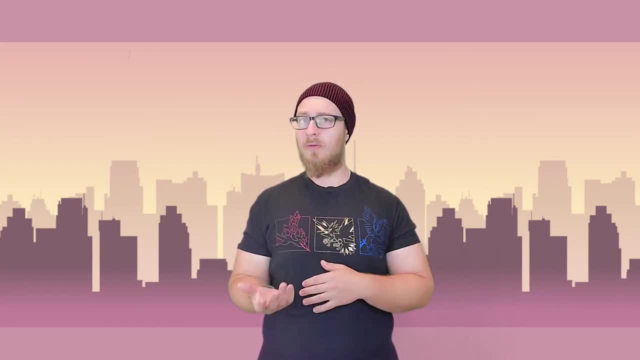 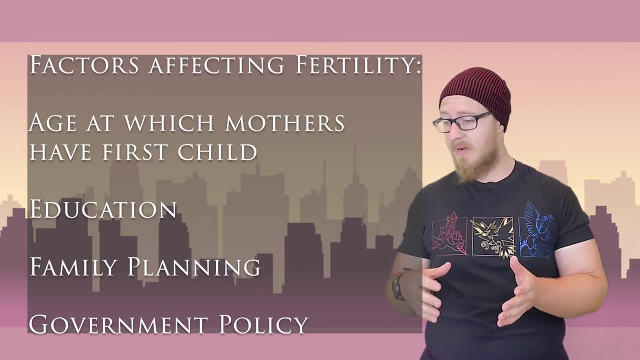 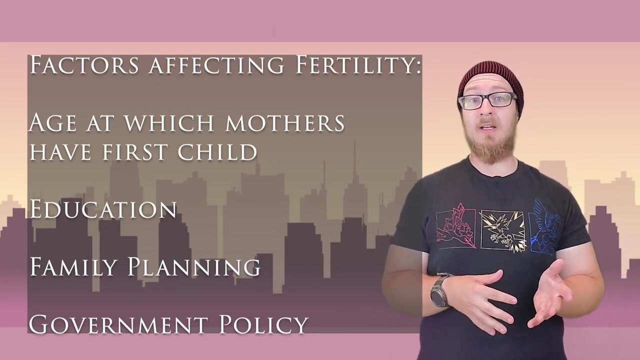 food has been increasing around the world. Healthcare is not the only thing that may affect the fertility rate, however. This is also impacted by the age at which mothers have their first child, educational opportunities, access to family planning and birth control and, of course, government policies. 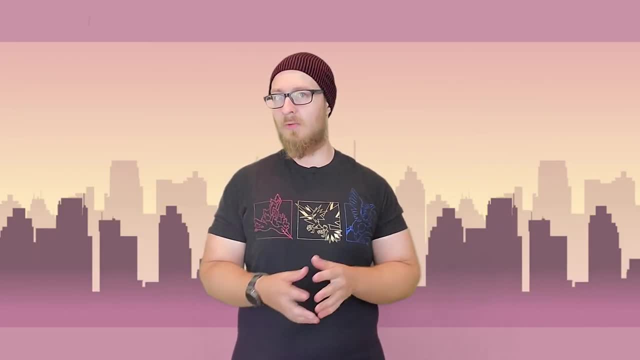 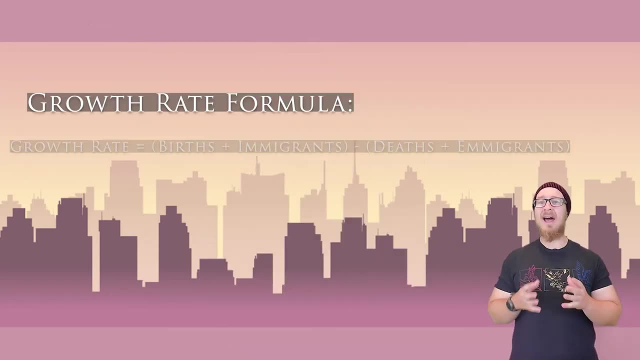 These birth rates are just one part of population growth. To get a full picture, we need to look at how population growth rates can affect child growth. If we are trying to frame our population's, birth can change. The way you calculate a population growth rate is you take the birth rate and the 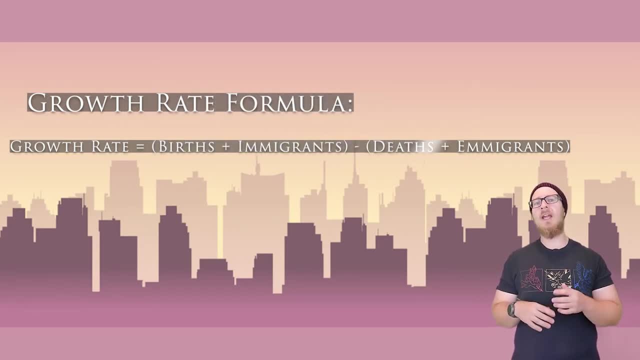 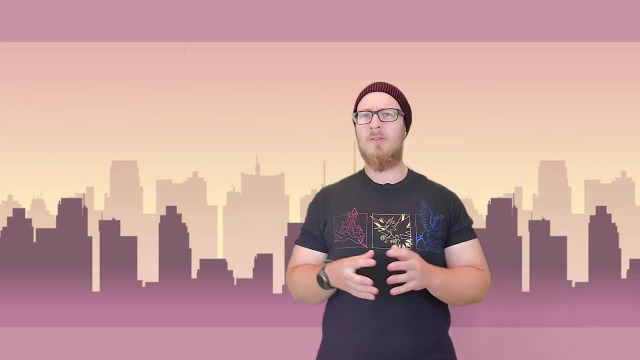 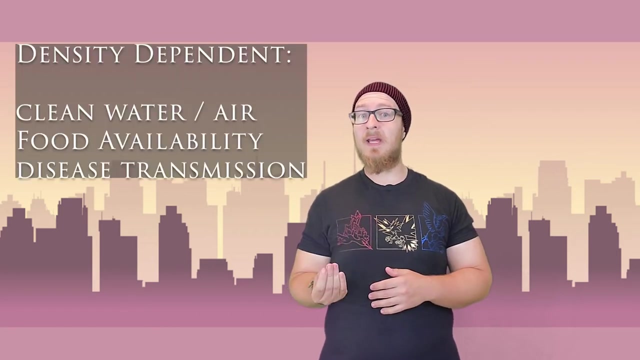 immigration rate into a region and subtract from that the death rate and the emigration rate, or how many people are leaving a region. Though the equation is self-explanatory, population growth can further be affected by density-dependent factors like access to clean water and air. 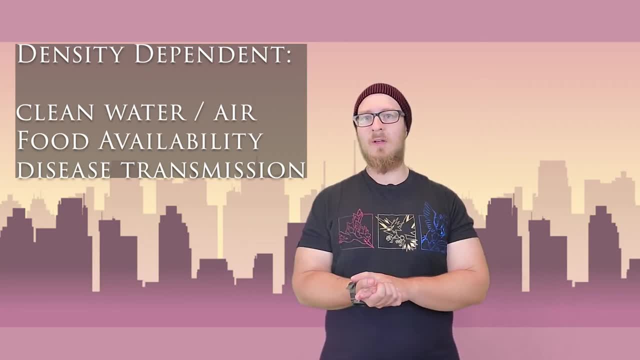 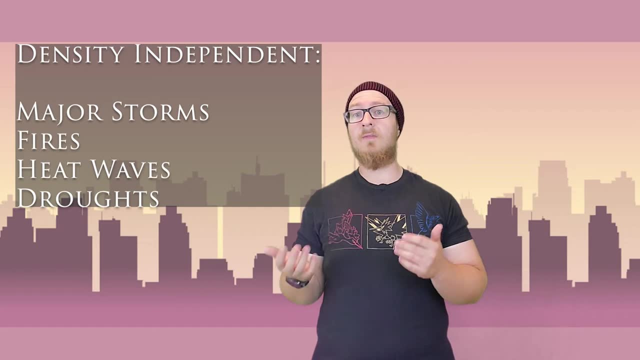 food availability and disease transmission rates. There are also the density-independent factors that may affect human populations, like major storms, fires, heat waves and droughts, and those aren't necessarily always calculated as part of the growth rate equation. Once you have a population growth rate, you can use that number to estimate the amount of time. 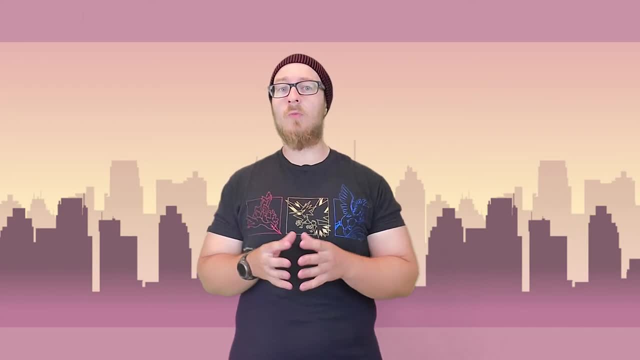 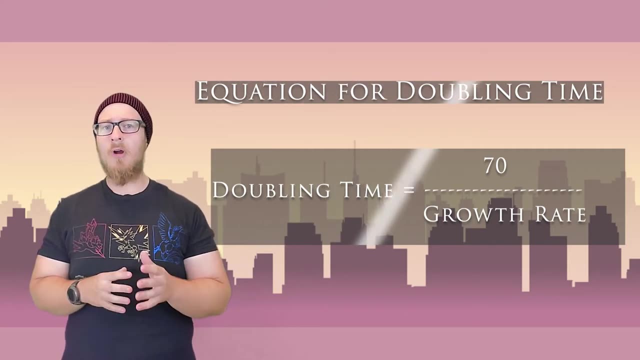 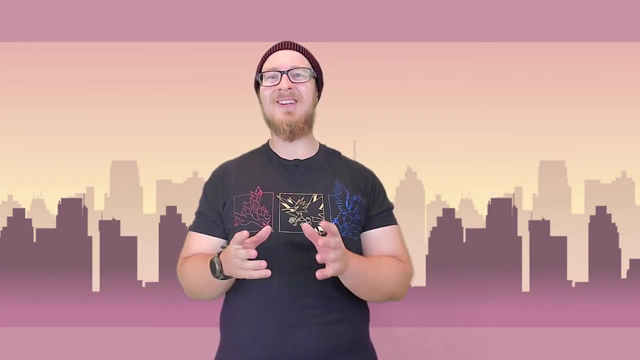 it would take a population to double in size using the rule of 70.. The rule of 70, states that dividing 70 by the population growth rate will approximate the amount of time it takes for a population to double. That sure is a lot of math. so let's take a look at a visual. 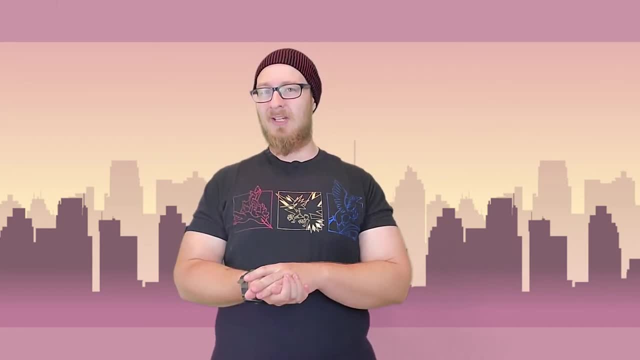 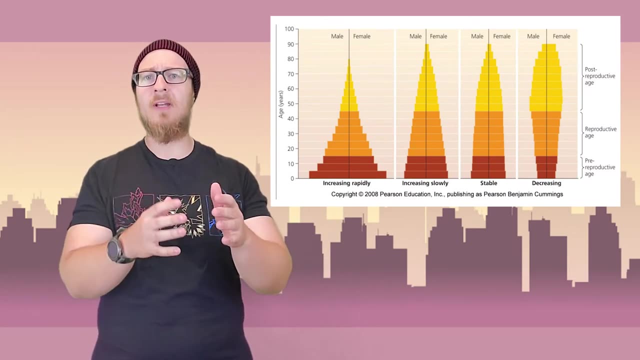 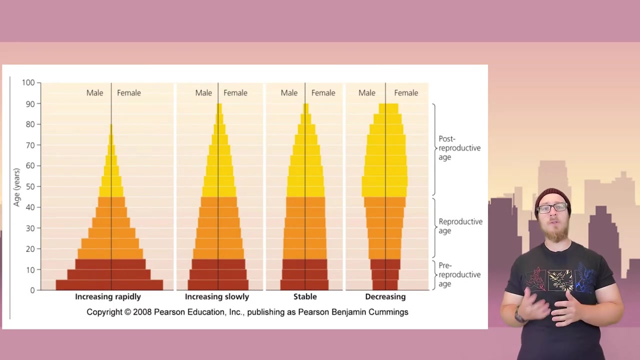 representation of how we can analyze human populations. Age structure diagrams are how we represent populations by cohorting them into age groups. In general, a rapidly growing population will have a higher proportion of young people than a population with a higher proportion of young people compared to stable or declining populations. The more children are born, the greater the future. 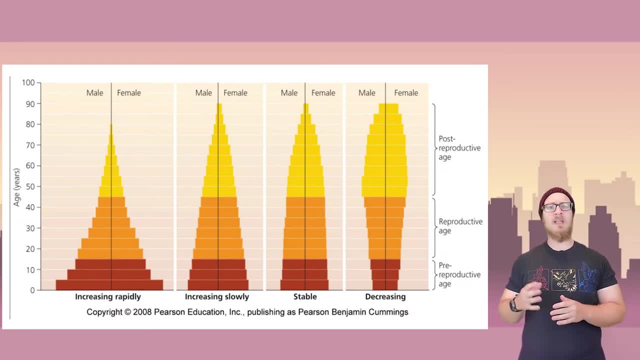 population will be. This is exemplified by the age structure diagram on the far left. A stable population will see about the same amount of children as adults. That's somewhere near the middle in the diagram, And for a decreasing population, the age structure diagram will. 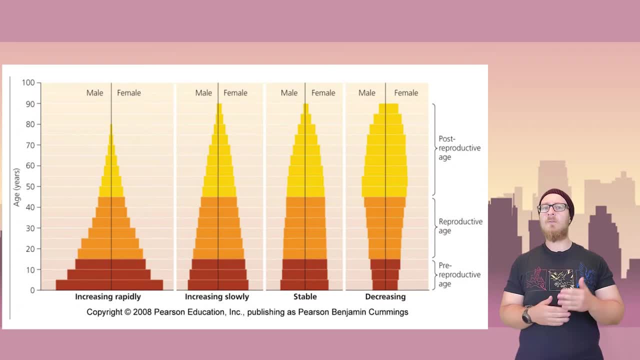 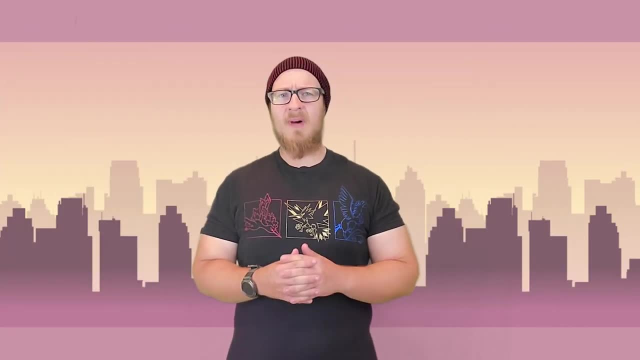 actually invert, It'll taper off at the bottom. So, for example, if you're a young person with a very small birth rate, you'll see a lot of young people at the bottom, as fewer children are born compared to the number of currently existing adults. These changing populations follow the. 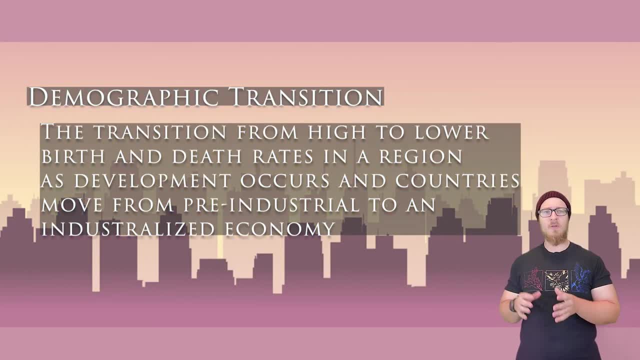 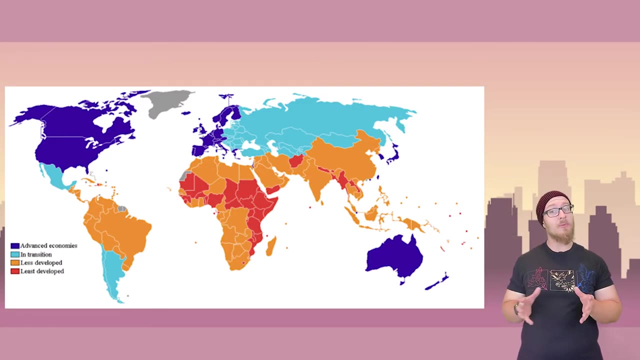 demographic transition or the transition from high to lower birth rates and death rates in a region as development occurs and countries move from pre-industrial to an industrialized economic system. Every developed country has gone through this transition process and many countries are at varying stages of this demographic transition. In AP Environmental Science, we use the four-stage. 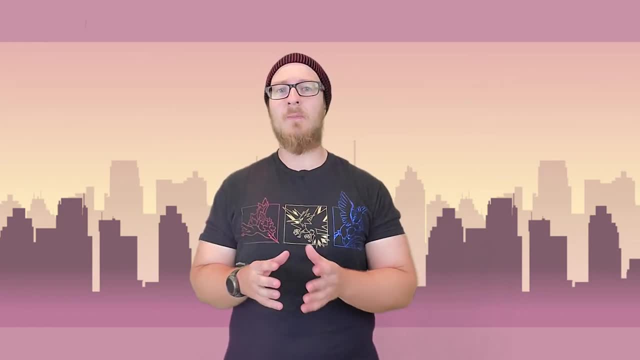 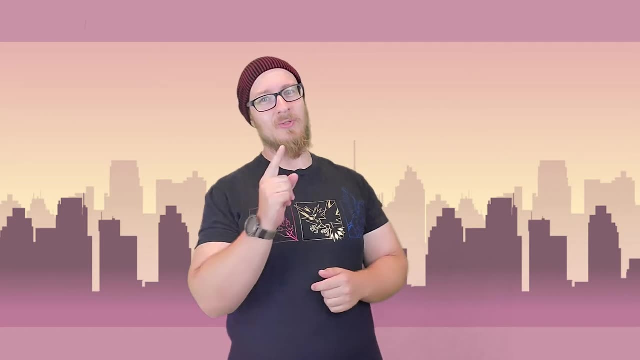 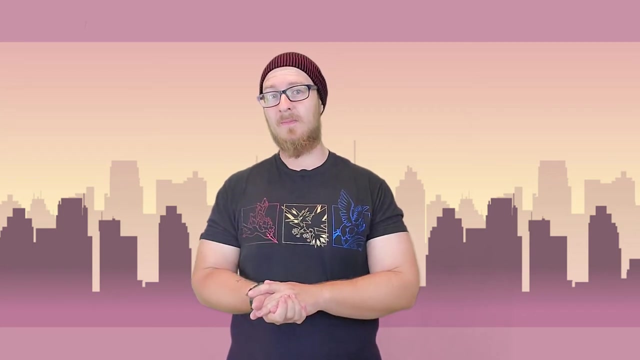 demographic transition model. So if you took AP Human Geography, do watch out, because that class uses a different model. So, yes, you still need to pay attention in this class, even if you are an expert in human populations from that class. Here I have represented the birth rates in pink: the. 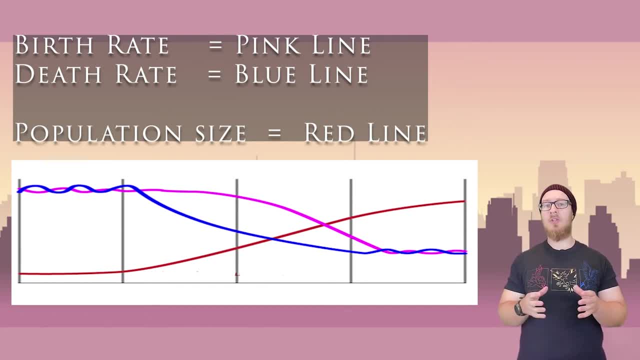 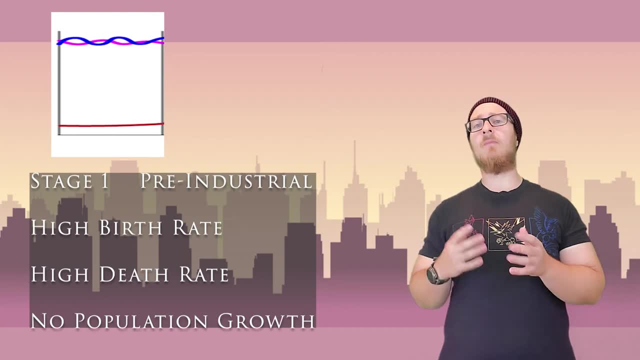 death rates in blue and the total population in red. A stage one or pre-industrial society will see high death rates and high birth rates with very little population growth. This is generally because having many children is the norm but because of high infant mortality, many do not make it to adulthood, so the population doesn't really grow. A stage two or developing country will continue to have a high birth rate and very little population growth. but because of high infant mortality many do not make it to adulthood, so the population doesn't really grow. 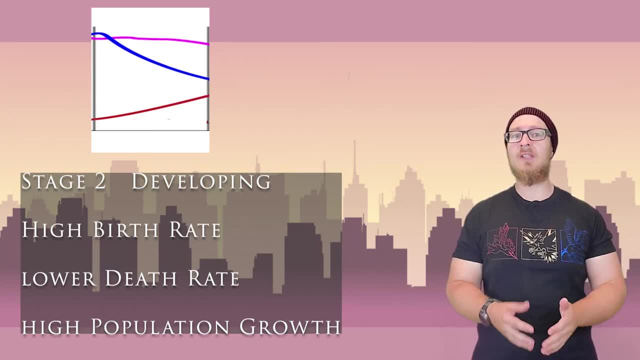 A stage three or pre-industrial society will continue to see high birth rates, as children are necessary economically speaking, but death rates begin to decrease due to improved health care and sanitation. Here is where we begin to see a spike in population growth. 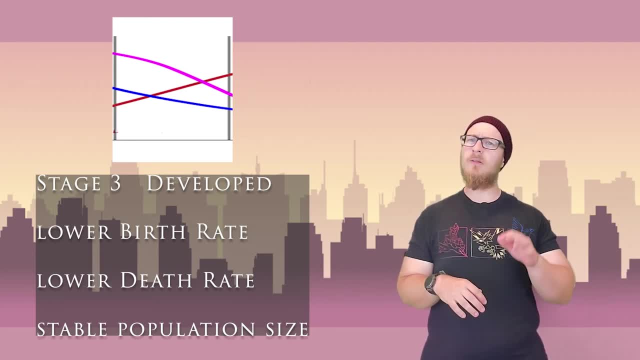 A stage three or developed society will see lower birth rates and low death rates. This is because of an increase to access in health care and family planning. In developed countries, a greater amount of women opt to have fewer children because of careers and access to education. 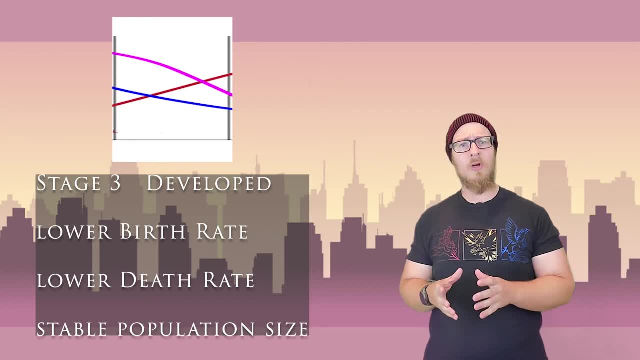 opportunities. Death rates are also low because there is now an established medical infrastructure In a developed society we start to see a very stable population. Perhaps it's increasing slightly, but the numbers of people more or less stay about the same: A stage four or post-industrialized country.